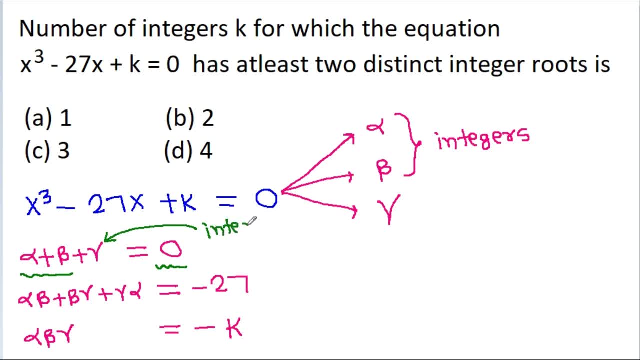 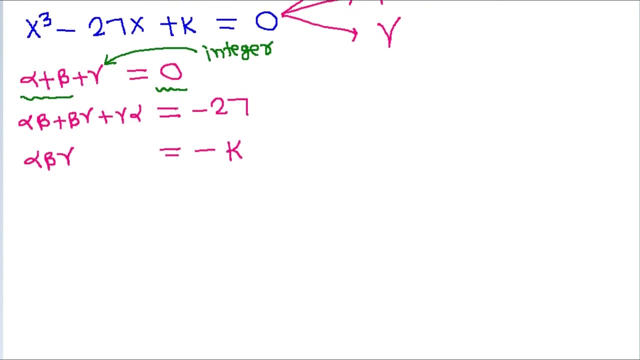 So we get gamma also must be integer. So we get: all three alpha beta gamma are integers. But we have to keep in mind that all three alpha beta gamma cannot be equal, Because we have given at least two distinct integer roots And we have anpha plus beta plus gamma is equal to. 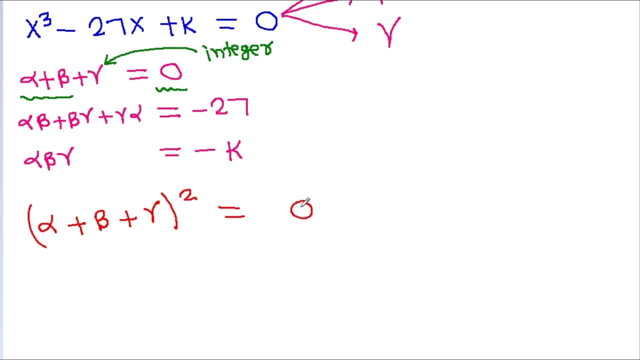 zero. and if we square both sides, then we get anpha square plus beta square plus gamma square plus two times anpha, beta plus beta, gamma plus gamma. anpha is equal to zero. Or we get anpha square plus beta square plus gamma square plus two times anpha, beta plus beta gamma. 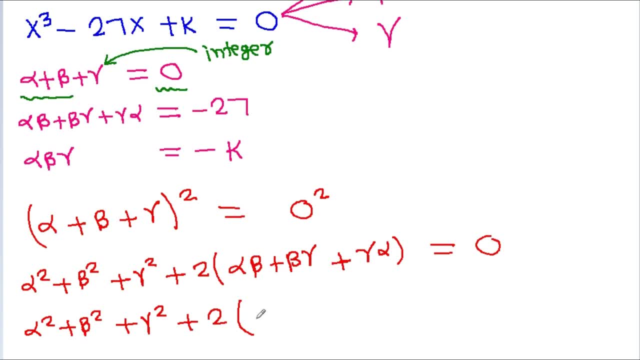 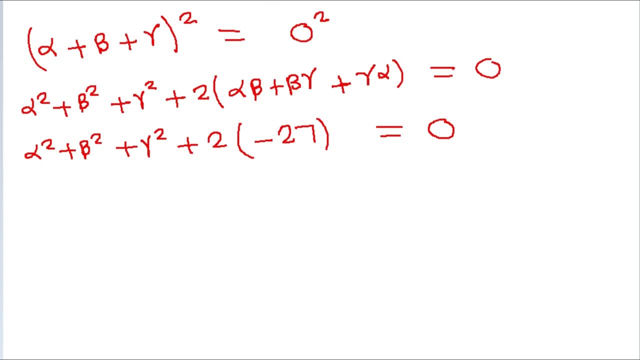 plus gamma anpha is equal to minus 27. it is minus 27, that is equal to zero. And get alpha square plus beta square plus gamma square is equal to 2 times 27, is 54 and we have alpha, beta, gamma are integers. so the possible squares are 0, square is 0, 1 square is 1, 2 square. 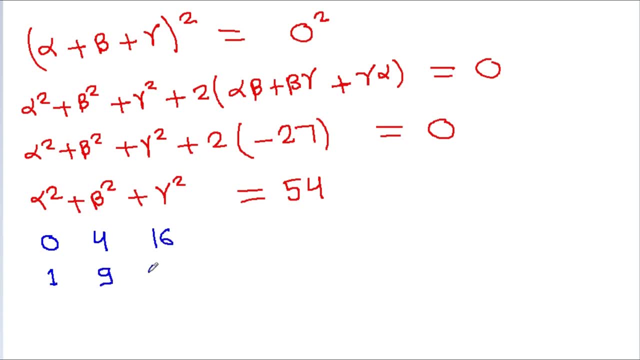 is 4 and 9, 16, 25, 36, 49 and next 64 will be greater than 54. and we can also check parity. we have: alpha plus beta plus gamma is equal to 0 and alpha square plus beta square plus gamma square. 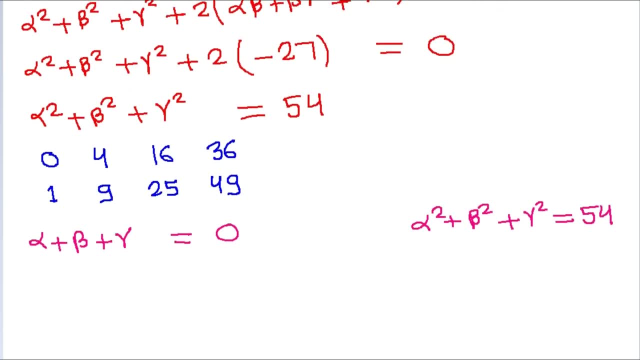 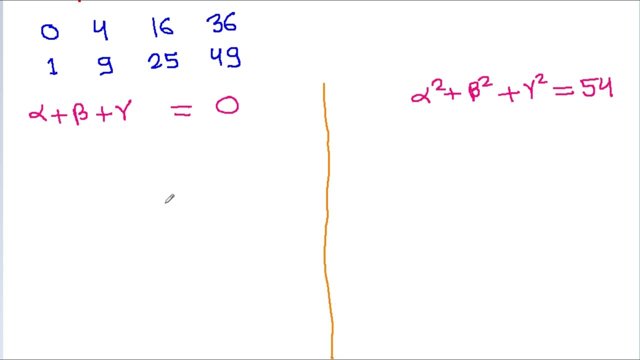 is equal to 54 and the possible cases are: alpha beta gamma can be even, even, even or two is odd and one is even, or one is odd and two is even, and we have: sum of alpha beta gamma is equal to zero, that is even, and sum of one odd and two even is odd. so this case is not possible. 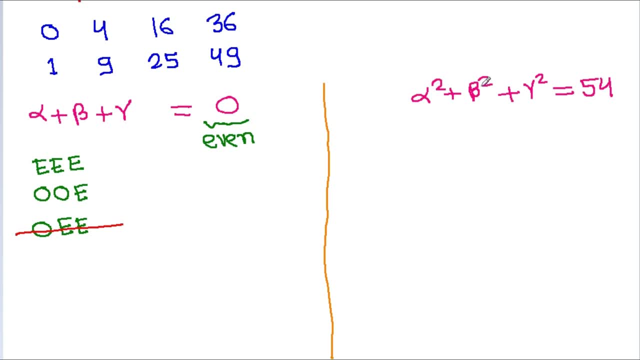 and now we have alpha square plus beta square plus gamma square is equal to 54, and we know that even square is in the form of 4k and odd square is in the form of 4k plus 1, and 54 is not a multiple of 4, so all three cannot be even, so this case is also not possible. 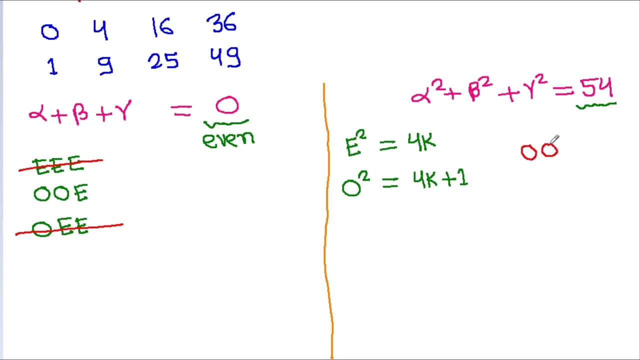 so alpha, beta, gamma are odd, odd and even, and we have values for alpha square, beta square and gamma square. these are even values and these are odd values. so by hit and try method, if we start with 49, then if we take 1 and even 4, 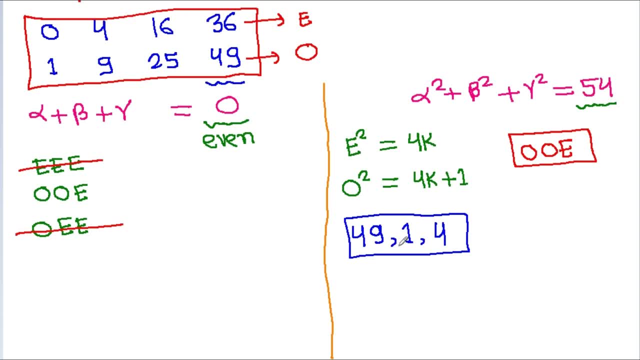 then the sum will be 54 and in this case the numbers will be 7, 1 and 2 and from 712. in any way we cannot get alpha plus beta plus gamma is equal to zero from 712. 7 plus 1 minus 2 is also not equal to 0 minus 7 plus 1 minus 2 is also not equal to 0. 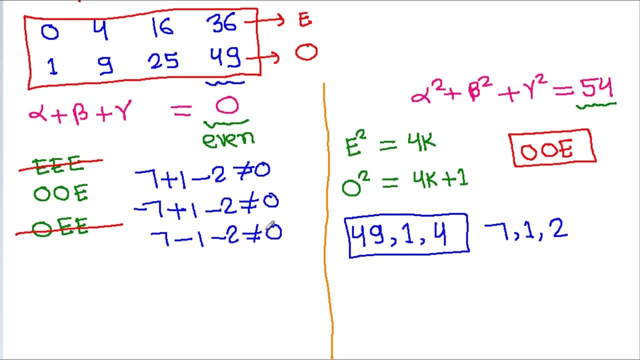 7 minus 1 minus 2 is also not equal to 0, so from 712 we cannot get. alpha plus beta plus gamma is equal to 0. so this is not possible. and now if we start with 25, then if we take 25 and 4, then the sum will be 54 and in this case the numbers will be 5, 5 and 2, and from 552. 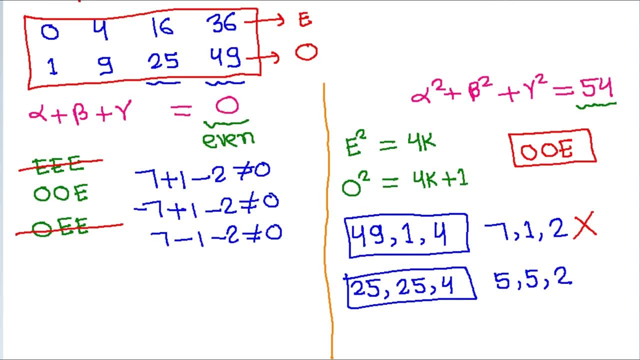 also, we cannot get: alpha plus beta plus gamma is equal to 0. so this is also not possible. and now, if we start with 9, then if we take 9 and 36, then the sum is 54, and in this case the numbers are 3, 3 and 6, and from 3, 3, 6.